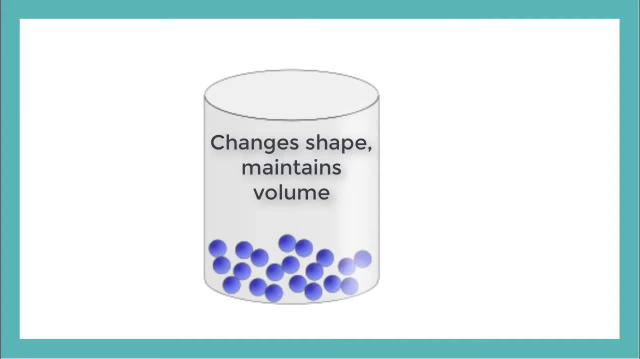 Liquids are able to flow and change their shape because their atoms and molecules are not fixed. They can slide past each other. Gases are made up of matter with no specific volume or shape. Gases will take up as much space as they can, filling any container. 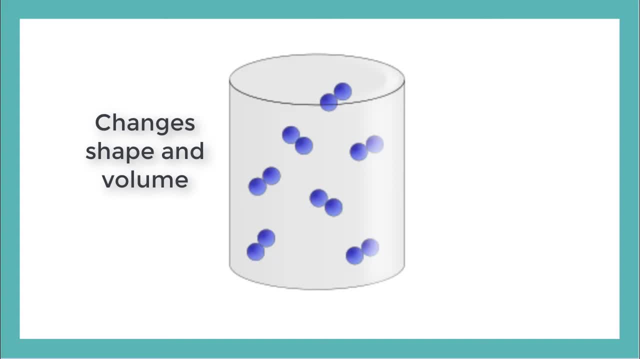 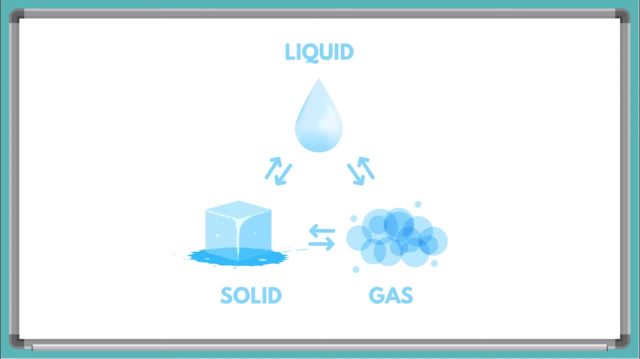 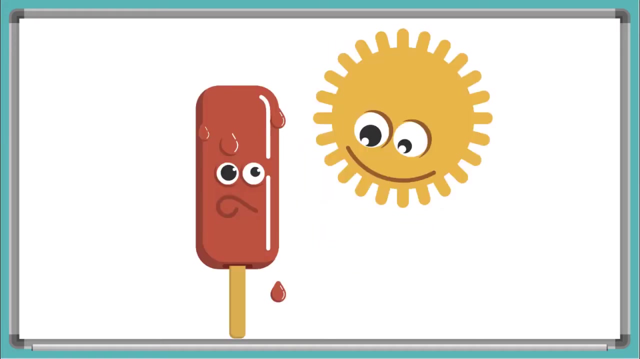 Gases are able to change their shape and their volume because their atoms and molecules move freely and quickly. We can change the state that matter is in. This is called a transition. A transition is when a substance changes from one state to another, like a chocolate bar turning into a chocolate puddle if left out in the sun. 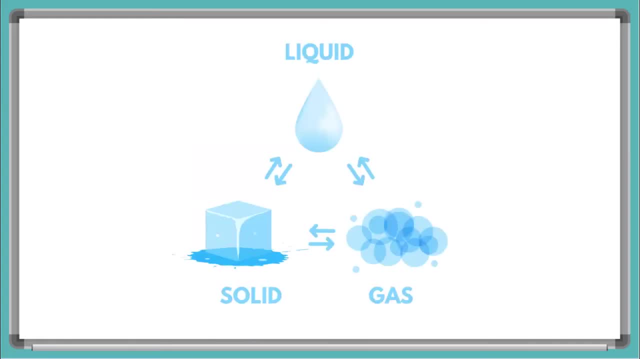 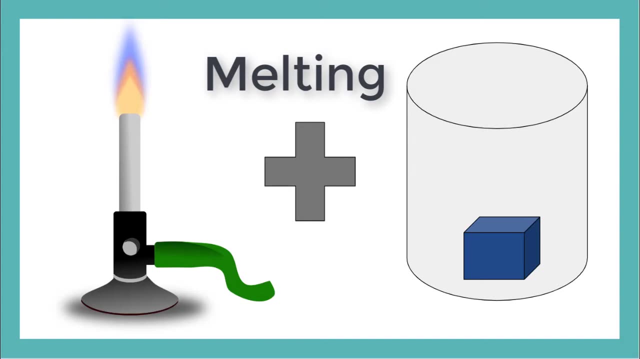 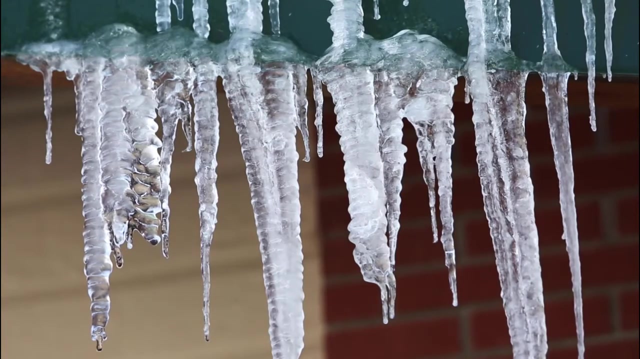 There are four types of transitions. The first one we will talk about is melting. Melting happens when heat is applied to a solid and it transitions to a liquid, Like icicles, which are made of solid ice, melting into liquid water as the day warms up. 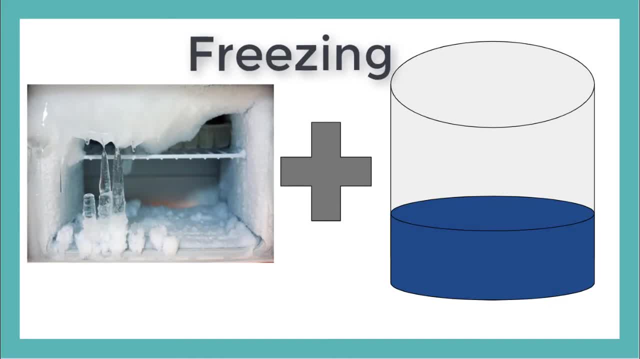 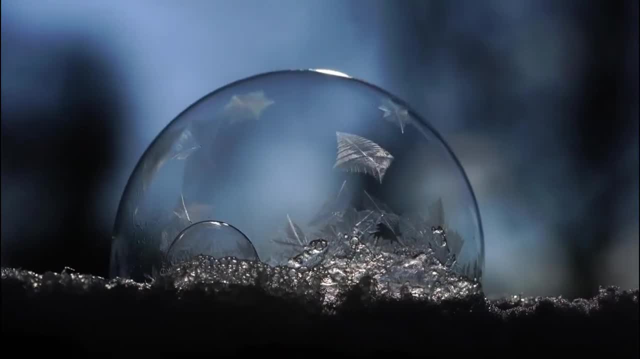 The next transition is freezing. Freezing happens when extremely cold temperatures are applied to a solid. Freezing happens when extremely cold temperatures are applied to a solid. Freezing happens when extremely cold temperatures are applied to a solid. Freezing happens when extremely cold temperatures are applied to a liquid and it transitions to a solid. 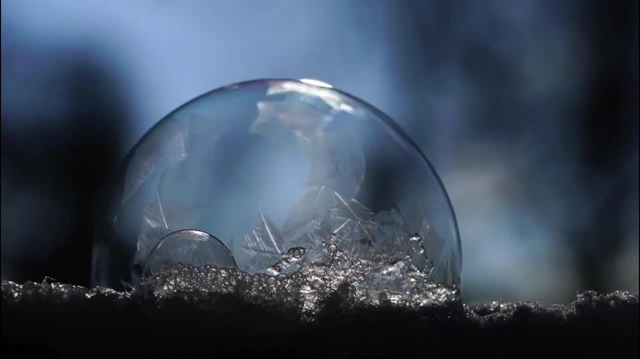 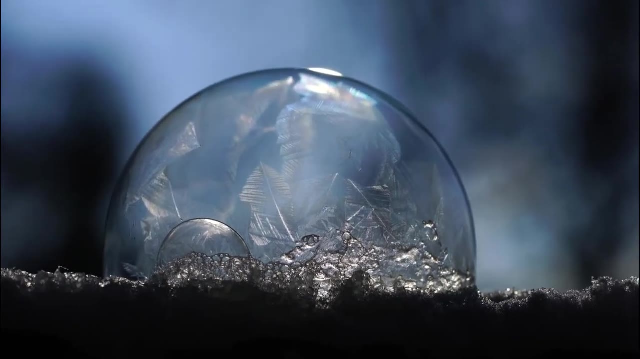 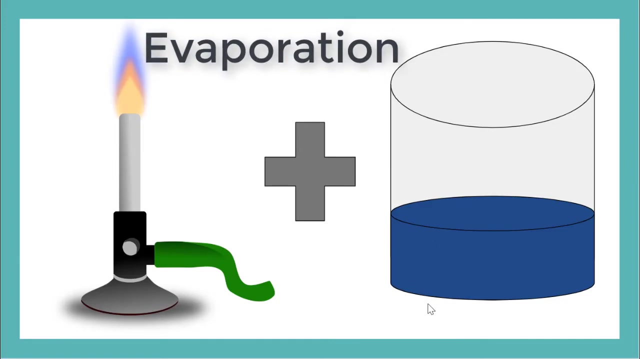 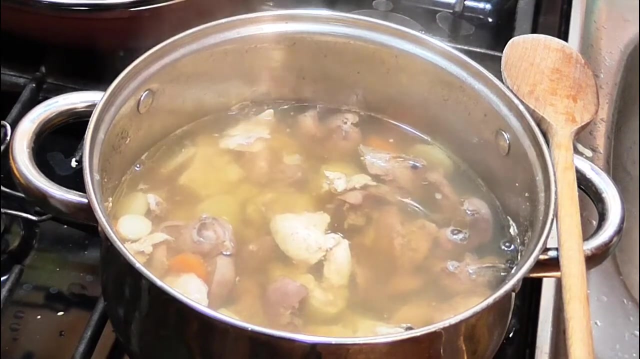 As you can see here, this liquid soap bubble becomes a solid in the freezing temperatures. Evaporation is another transition. Evaporation happens when heat is applied to a liquid and it transitions to a gas. The broth in the soup evaporates into steam when put on the stove to boil. 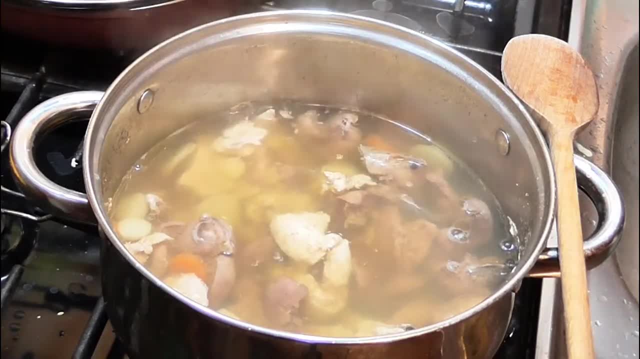 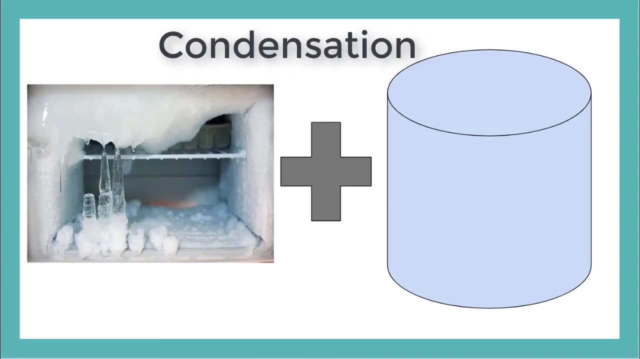 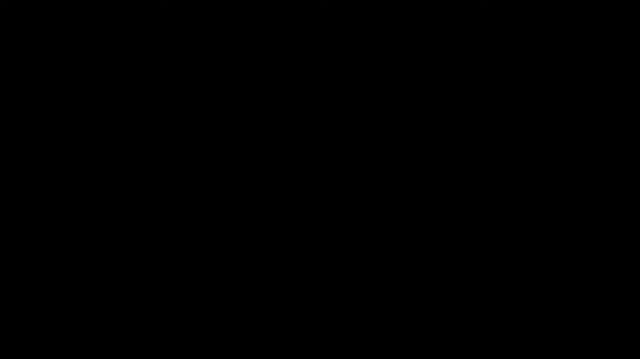 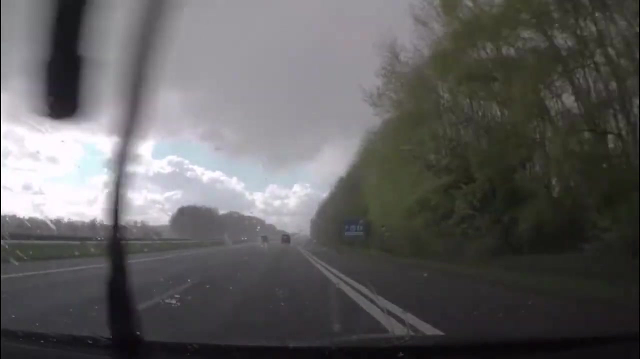 It's important to mention, though, that you can't actually see. the steam Condensation is the last transition. Condensation happens when cold temperatures are applied to a gas and it transitions to a liquid. Condensation happens when clouds full of water vapor are cooled to their dew point and produce rain. 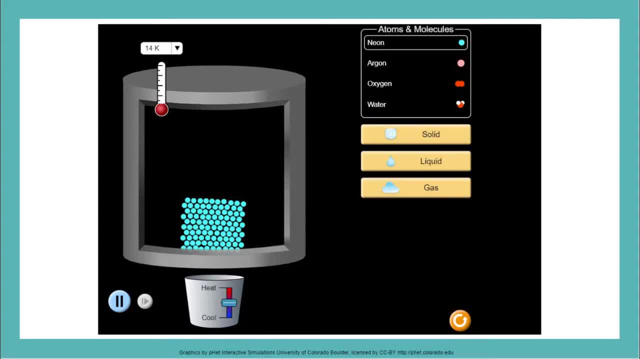 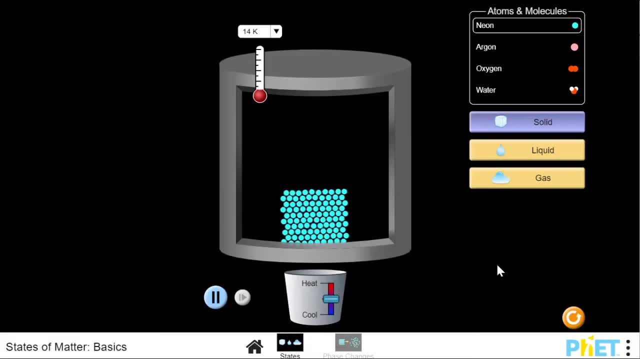 Repeat this process 4 times When it's destiny. fallballs appear, the particles are going toности will start moving forwards lately and they will be formed by a reaction from the bra, but actually leaving a solid, And then you will start the process of generalization. 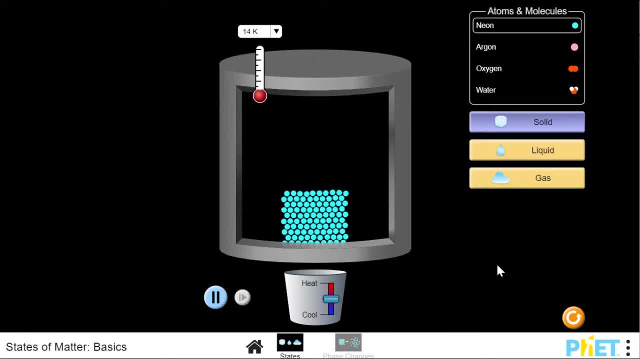 extreme temperature waves and loses in as surprise as possible, but for extreme temperatures they are somewhat irregular. Now that we know about the fourth transition, let's see what the particles look like in each state. Let's jump into a fete game. Here we are in the fete game called states of matter, basics, and we are in the first game called states. Just to show you around, here's our container, Here is our atoms or molecules. you can choose of these different atoms and molecules over here, And we also have a heat lever here that I could drag this blue bar up to make it warm so it stays운데. 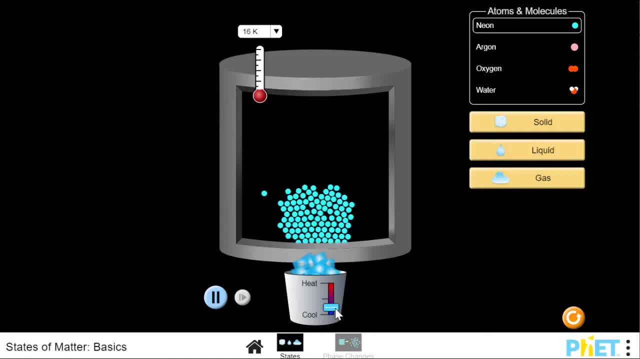 Shoot to include it warmer, or down to make it colder, And then I can also choose one of these here to automatically put the temperature that would make my atoms be in the state of solid liquid or gas. So let's just play around with this neon atom. We know that it's an atom and not a molecule. 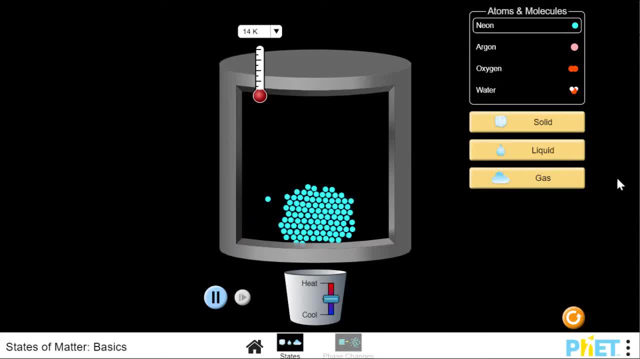 because it's just one. They're not bonded together. So I'm going to click on the solid button just to get started. So here we have a solid. They keep their shape and they have consistent volume. So what happens to a solid if I add some heat, So if I raise up my bar? 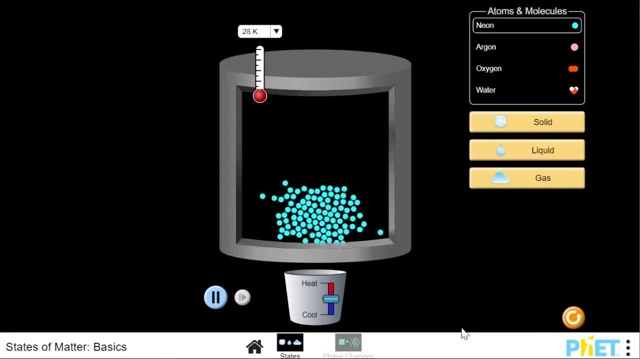 and I warm it up. what does it look like happened? They're moving around more. They're taking up more space. Overall, it looks like they're kind of taking up more space. So if I'm taking up the shape on the bottom here, this would give me the impression that I've melted. 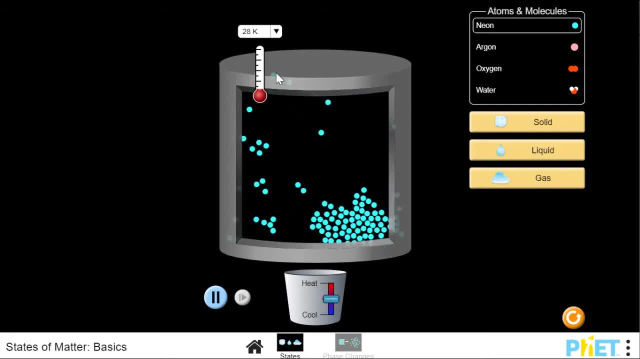 my solid neon into a liquid with a few particles that are acting like a gas. Now what if I click on the liquid? So this is what neon would look like as a liquid. So either I can heat my liquid and it would evaporate into a gas, or I can make it colder and freeze my liquid into a solid. 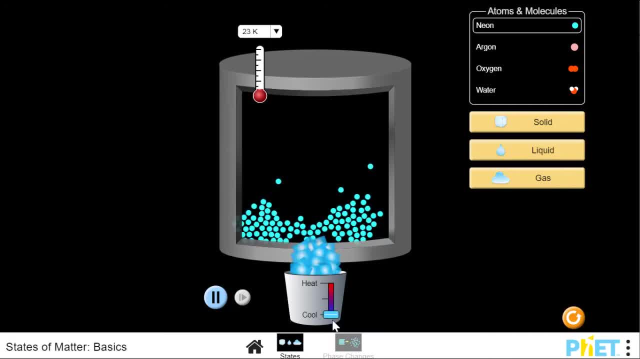 Let's see what happens If I cool it, So if I add some ice. so now I'm doing my freezing, So it looks like now they're all stuck in this new weird shape. Now what happened if I had neon gas? Click the gas here My temperature is the highest here.